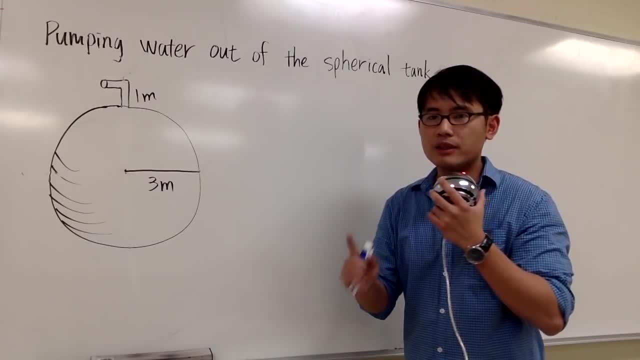 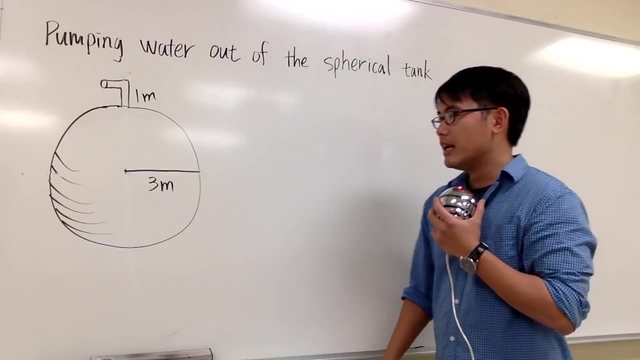 we need in order to pump out the water from the tank. the hardest part is we're going to draw a slice and then write an expression for the following slice. That's the hardest part, And let's see how can we do that. In order for us to do that, we of course have to come with 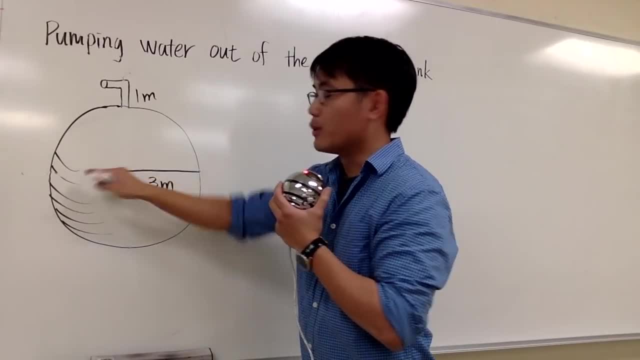 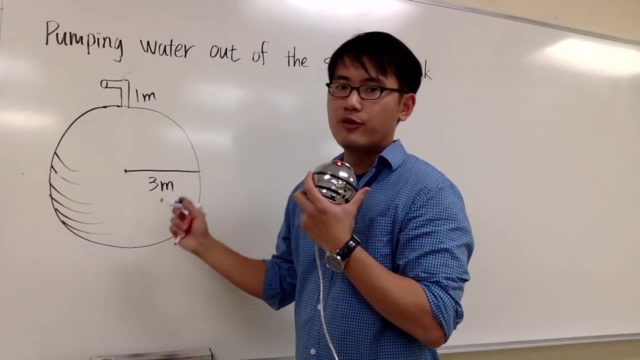 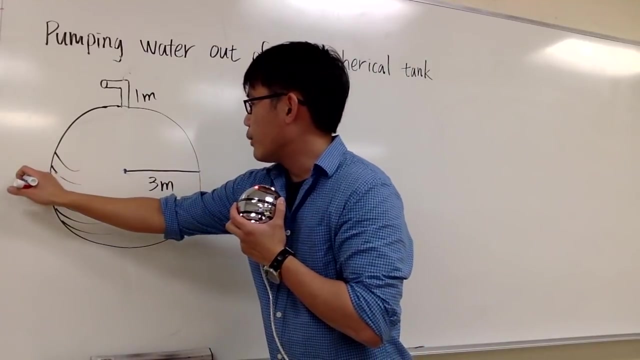 variables, especially because each average that will changes. we need to use equations, formulas and things like that, And- and I will pick a reference frame first- I will set up my x and y coordinate systems right here in the middle and I will just draw this right here as my x-axis. 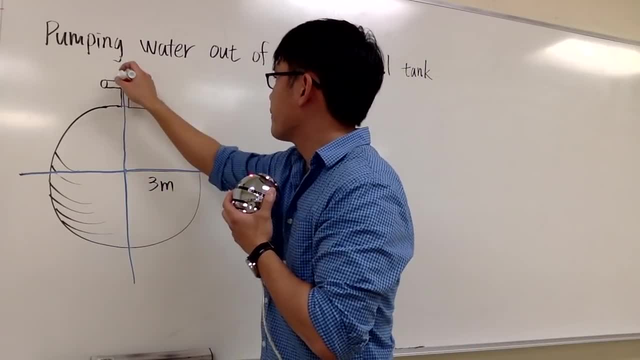 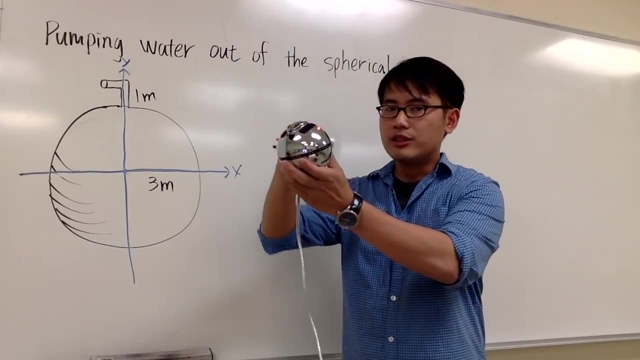 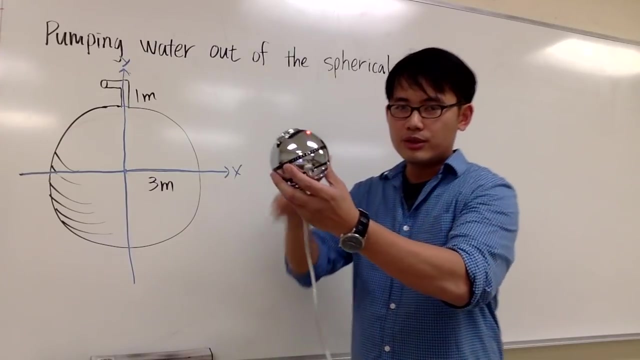 and then vertical as my y-axis. And now I have to ask you: imagine if you get a slice, just like cut through the slice of this sphere. what kind of shape are we going to get? So you can just look at the black part of the slice. 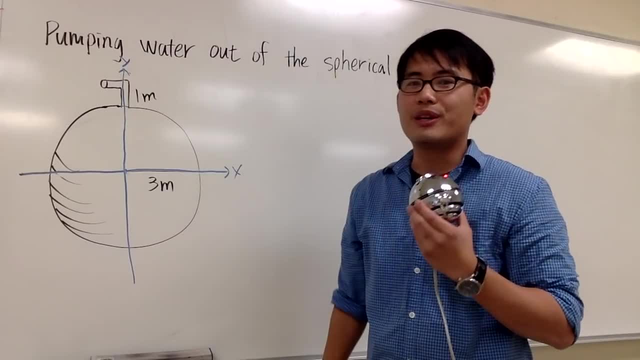 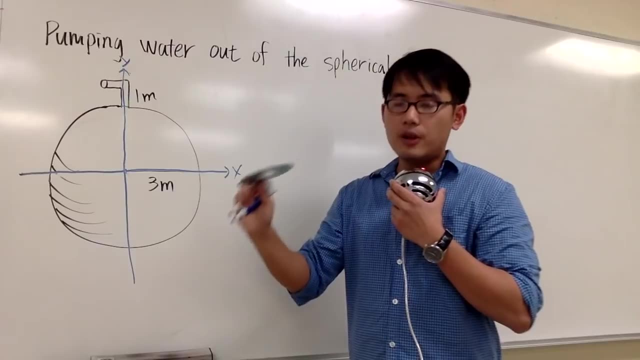 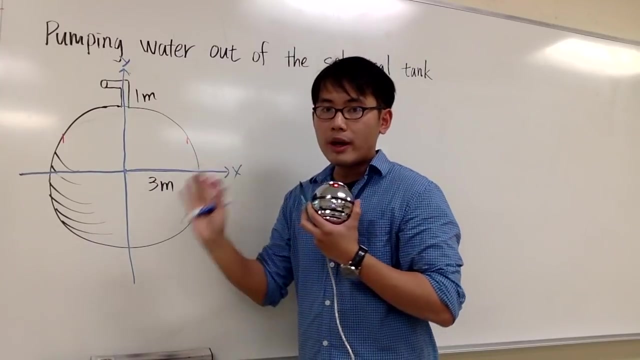 and just imagine if you just cut this piece out, what are you going to get? And the answer for that is: it's going to be like a CD, isn't it? So just remember, when you draw the slice, you have to look at what kind of shape. 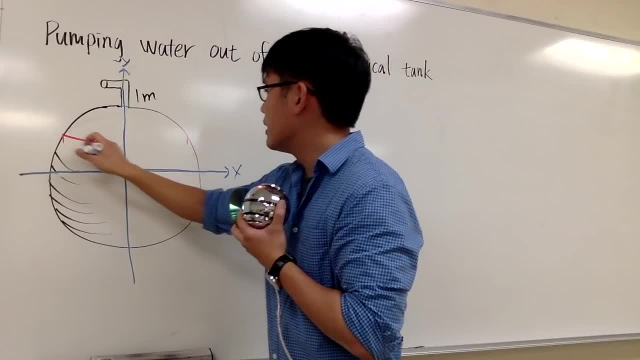 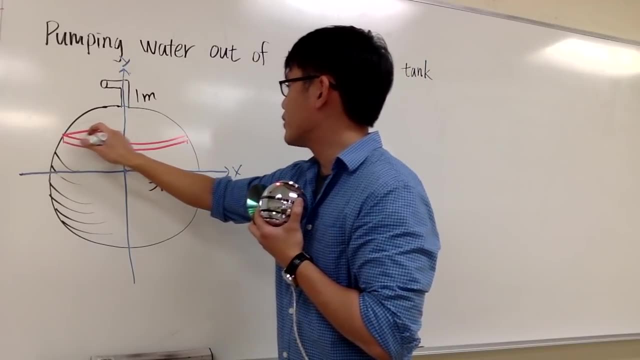 that you're going to get, And in this case we have pretty much a CD. And let me just draw the CD for you guys right here, And hopefully my picture is not too bad. So that's the CD I'm trying to draw. 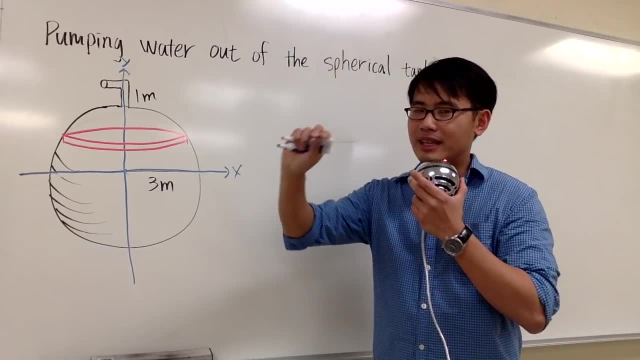 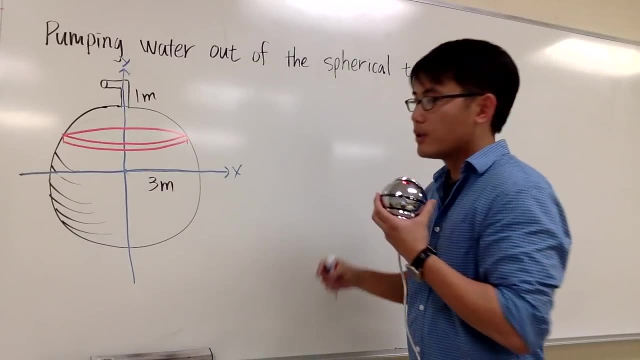 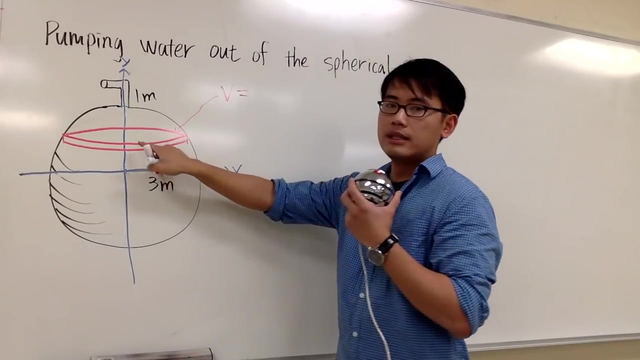 And then for CD, it's arguably a very thin cylinder, isn't it Right? If you make it more than that, Right? So now our goal, first goal is going to be finding the volume of this small cylinder, And this is in the shape of cylinder. 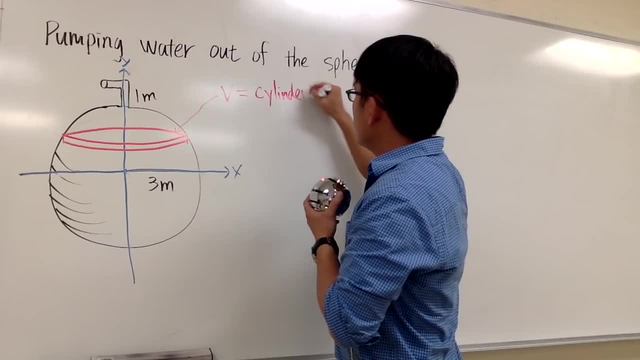 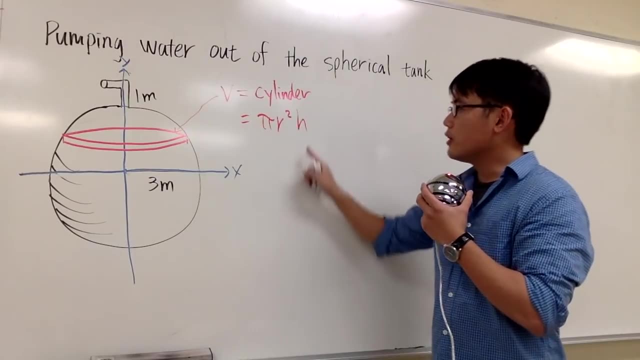 so, of course, let me write this down first: Cylinder, and the volume of the cylinder is just pi? r squared times h. So let's take a look. What's the height of this CD? Well, the height is right here. 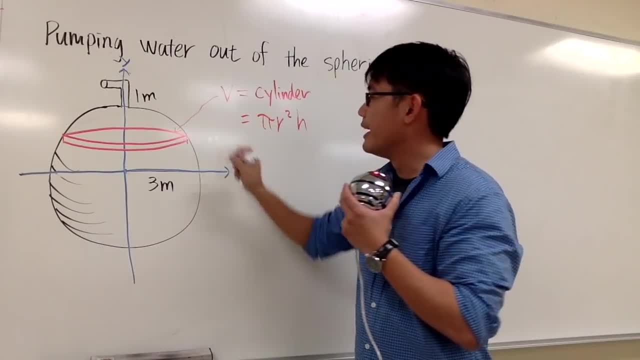 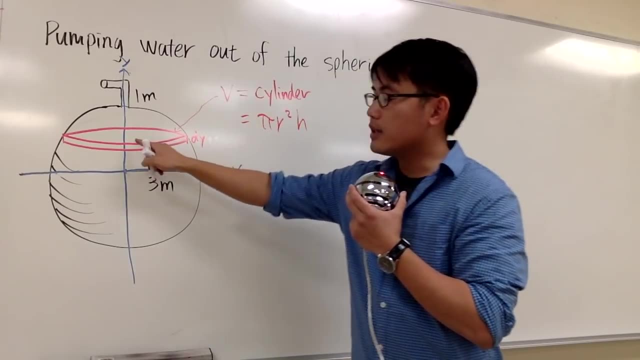 and then it's just going to be a small change amount in the y-axis. I will label this as the y and that will be for the h. And how about, in this case, what will be the radius? Well, for the radius. 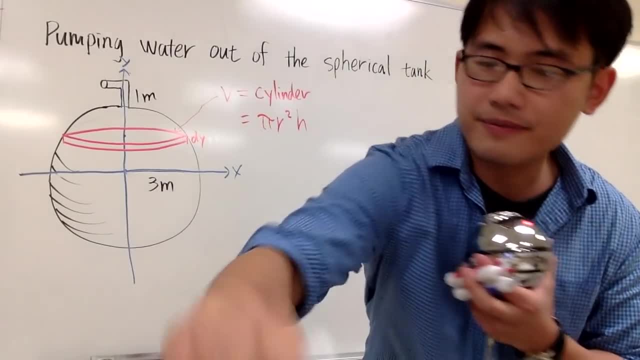 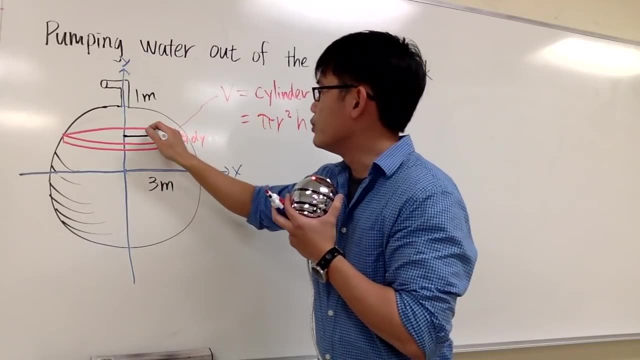 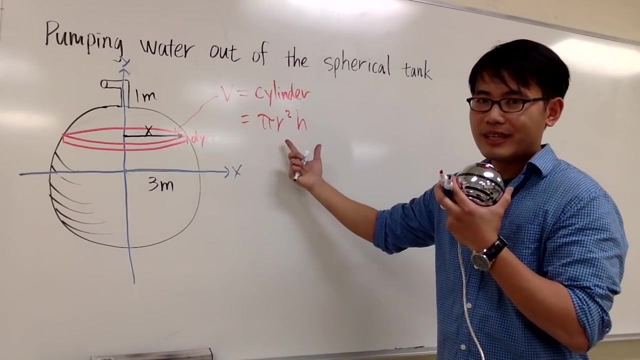 it will be just the distance from doing black. The radius will be just going from here to here And, as you can see, that's the horizontal distance which is the x-value. So I'm going to plug in x into the. x will be the radius. 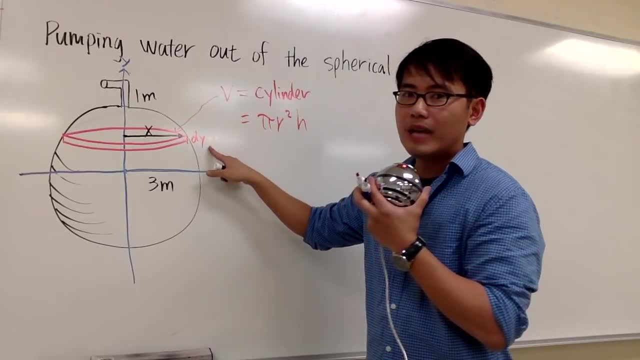 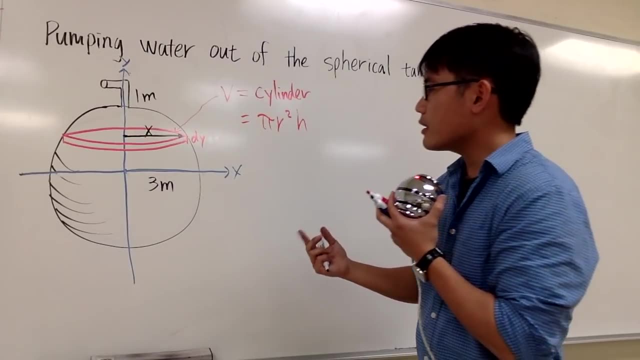 But then the problem is that the h is dy, so we have to be in the y-world in a minute. The x is going to be not so good, right? However, if you look at the part in black, we do have a shape that we know. it's a circle, right. 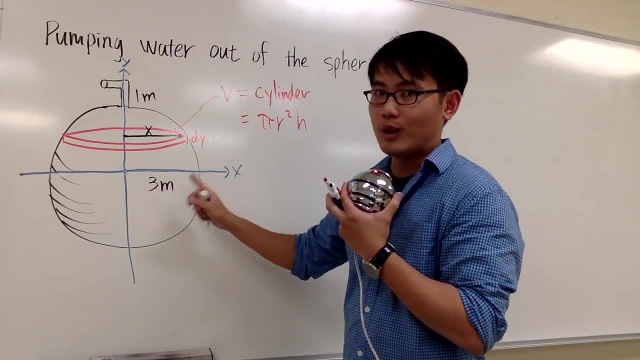 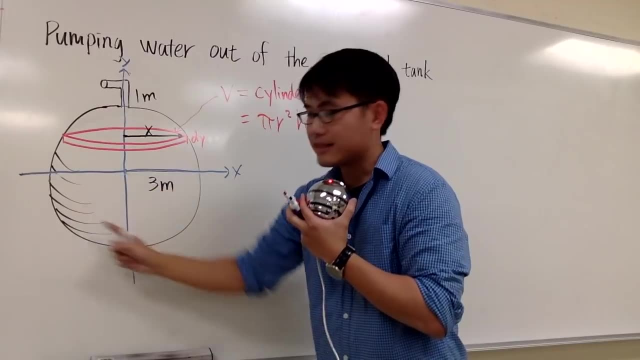 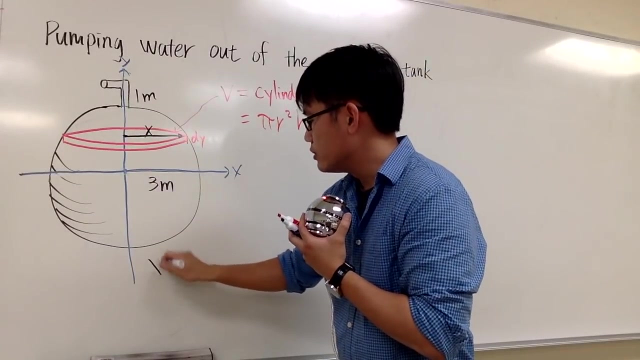 And then this right here was radius three. it was given earlier. Well, we can come with the equation, first based on the black circle right here and the reference spring. this is the center, as zero, zero. This circle has a equation. 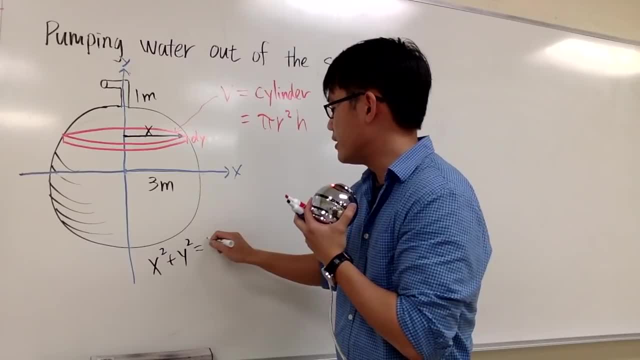 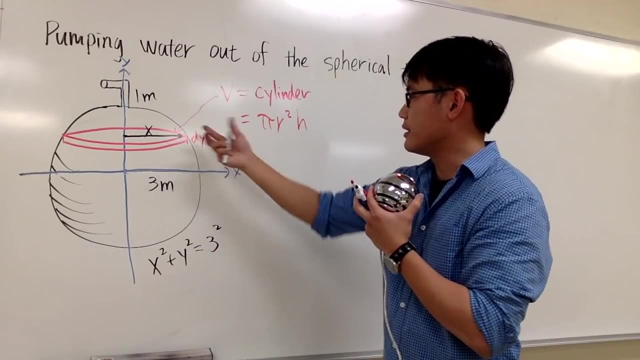 just x squared plus y squared equals to the radius, which is three squared, And I want to isolate that, And I want to isolate that, And I want to isolate that X, and that way I can plug in the expressions into the R, into radius, so I 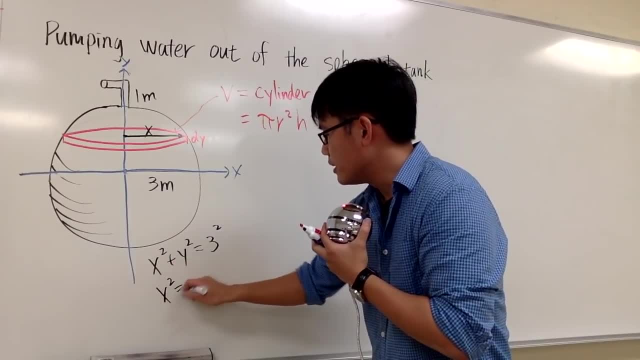 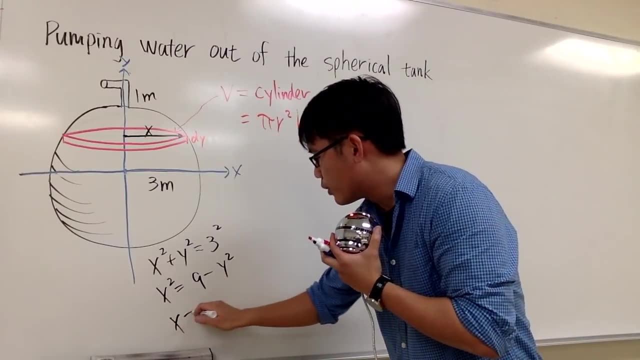 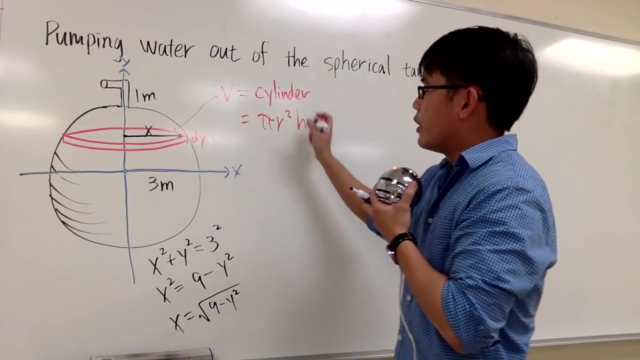 want to isolate X and you can see that X square will be: this is just 9, and then minus Y square, and I will take the positive square on both sides. in another word, X will be square root of 9 minus Y square. and now I can write an equation: 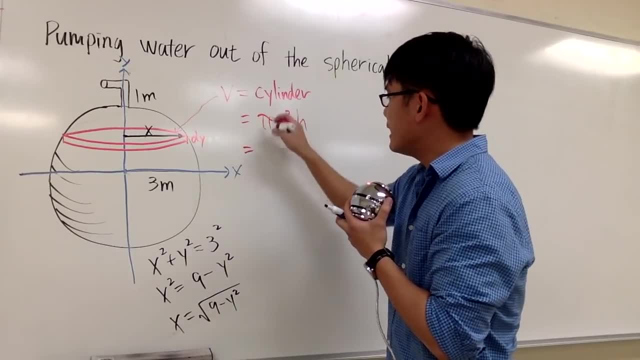 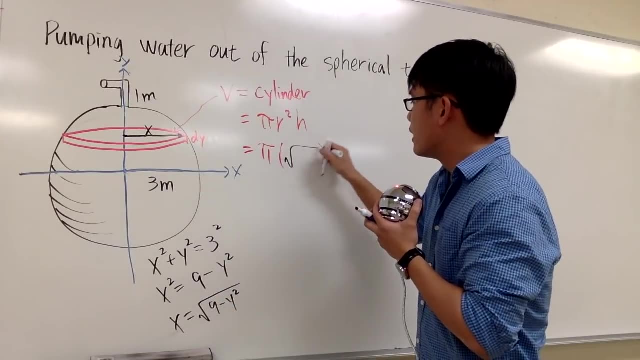 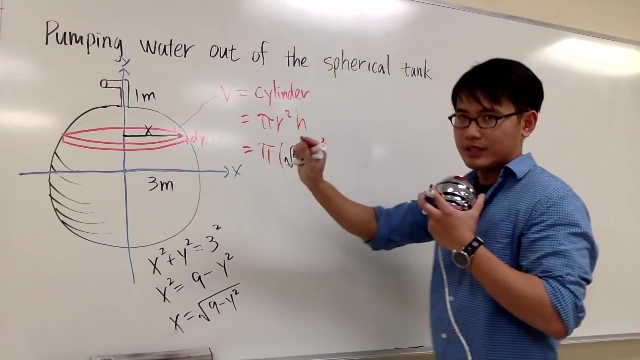 for the volume of this CD. PI is just a PI. the R is the X, which is that square root of 9 minus Y square, but then we have to square that, and then the H is the thickness with the height, which is the dy, and then pretty much that's it. 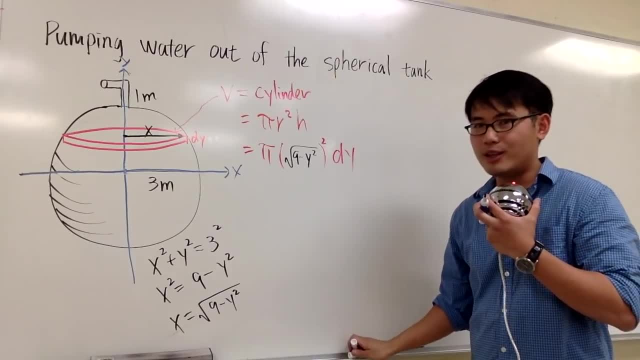 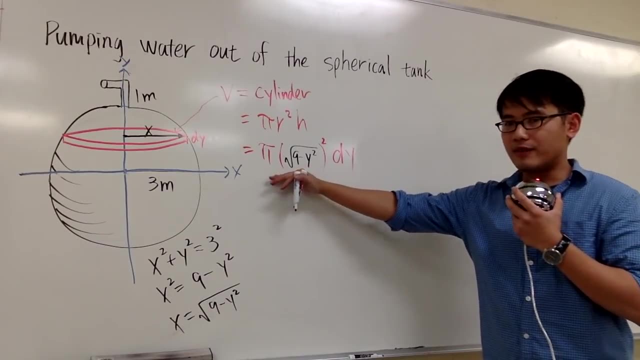 for the volume, and then we are ready to go to build out our integrals, to calculate the work that we need, and this is how we're going to do it. you let me just put this down first, and I will just write it down right here to. 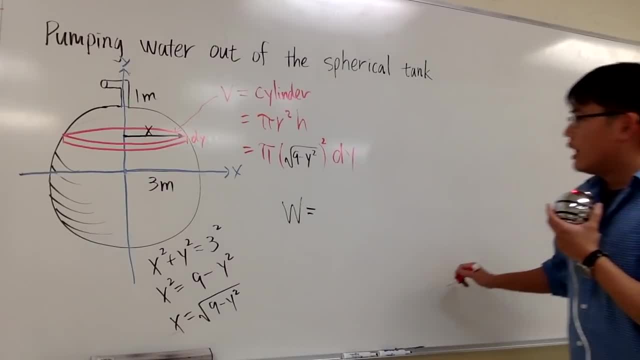 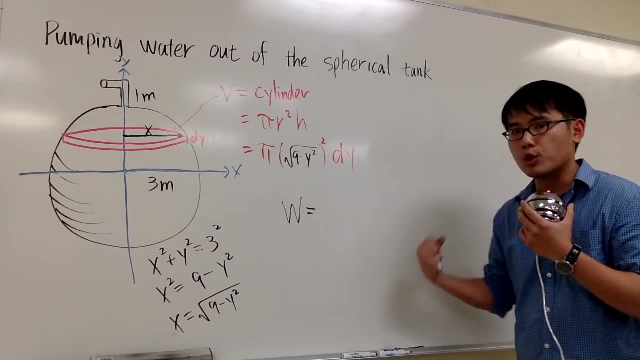 calculate the work. I want to write this down all the way at the end, because we have the dy and you know that we have to use integrals, so the dy should be all the way at the end and let me just write this down as pi and a square, square root. 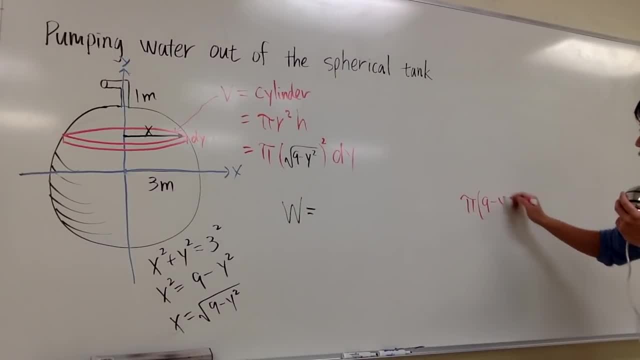 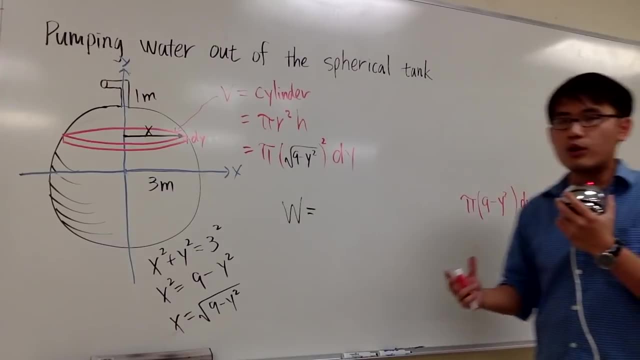 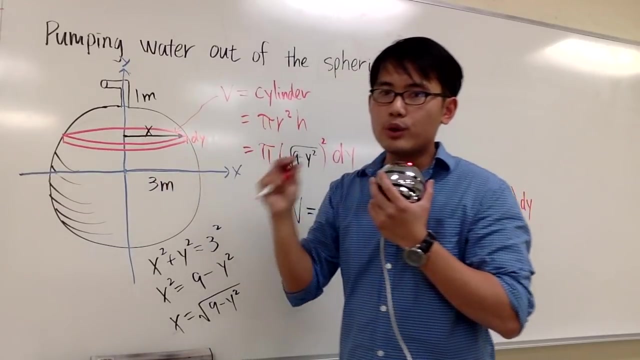 cancel. so let me just write it down as 9 minus Y square. then that's the inside right here, and then we have the dy all the way at the end. that's for the volume of this disc. and now you have to remember that this right here is filled with water, so we have to multiply by the volume the 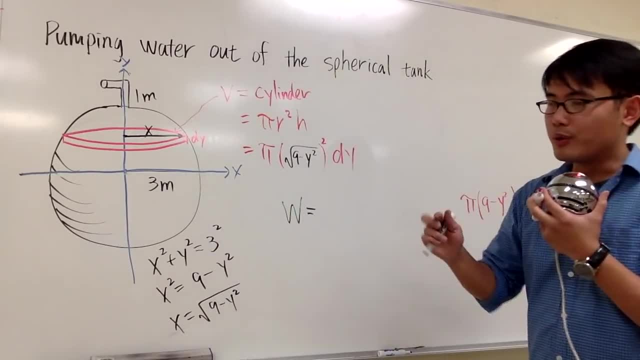 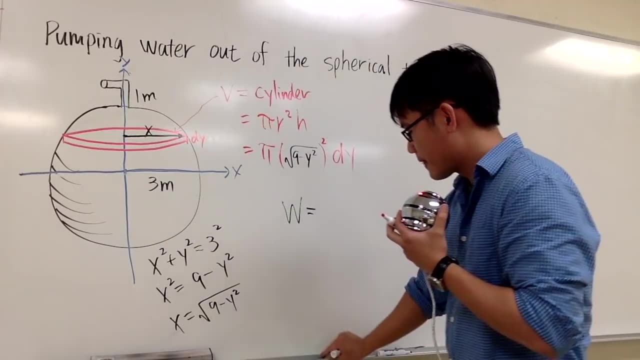 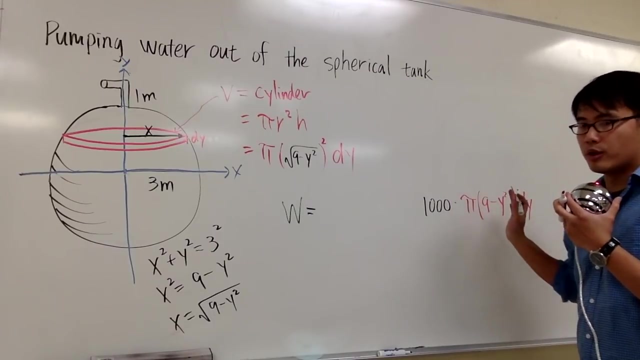 density of the water, because you have to. you pretty much try to find out how heavy. what's the weight of this disc filled with water? okay, and then the water density is 1000. so we will just multiply by 1000 in one of the units. by then we are in the Si units and right the meters. so I had 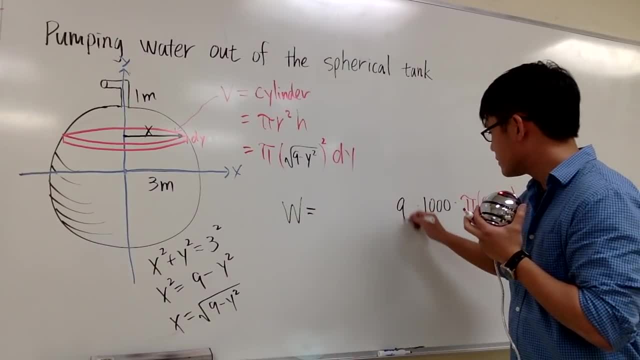 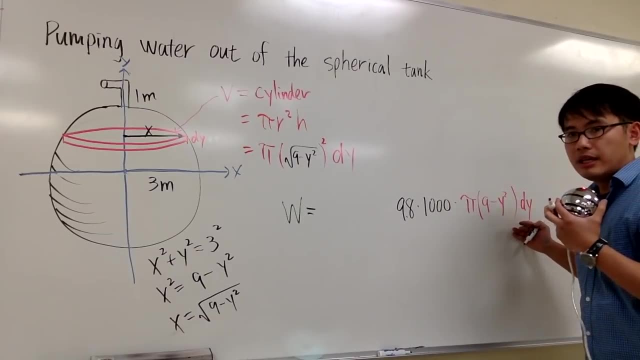 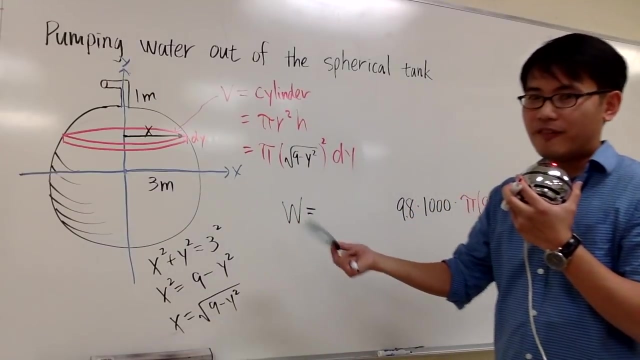 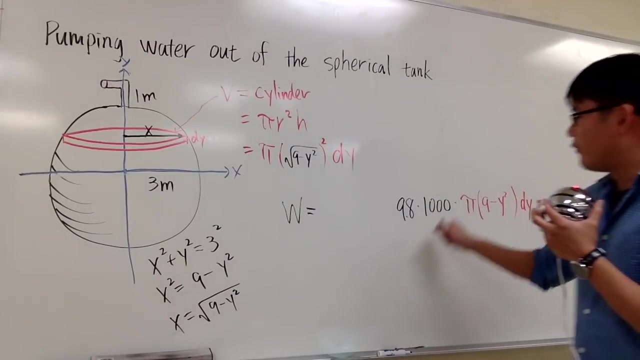 to multiply by 9.8 for the gravity. okay, so the water density in the gravity. so this right here represents the weight of this light of water and it's like that will be the force right, this right here is pretty much the force, and remember for the work is what force times distance i have to figure out. 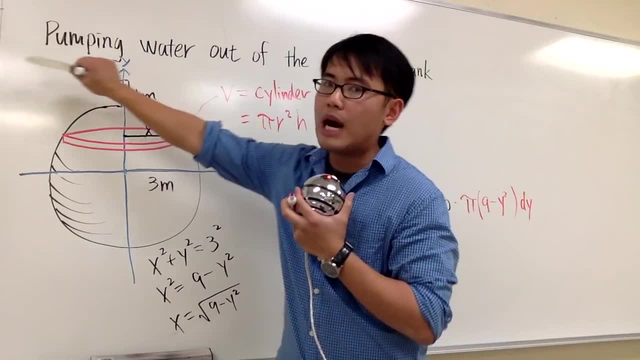 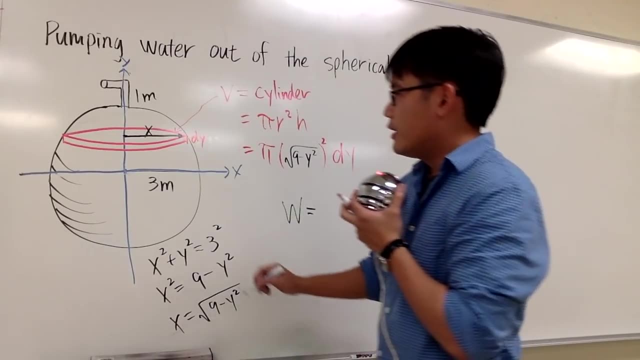 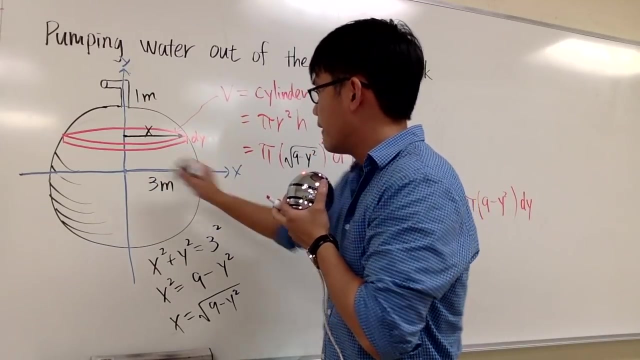 what's the distance that this cd has to travel in order to be out? right, that's the next thing i want to do, and then this is the part that requires more geometry. all right, i call this to be x, and then, on my coordinate system, of course, um, from here to here will be y, no problem. 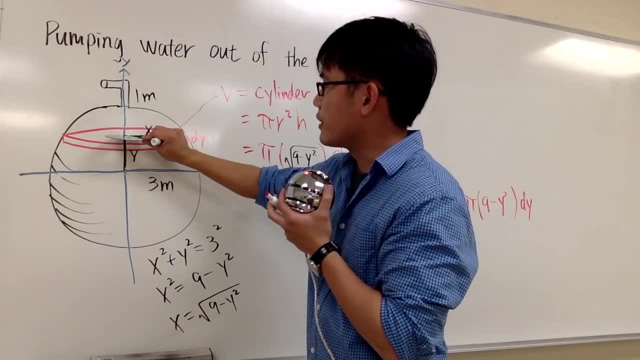 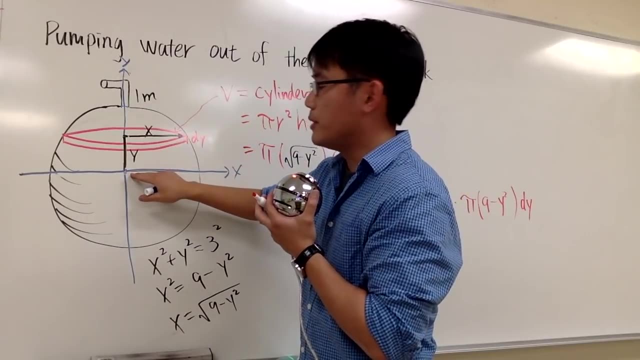 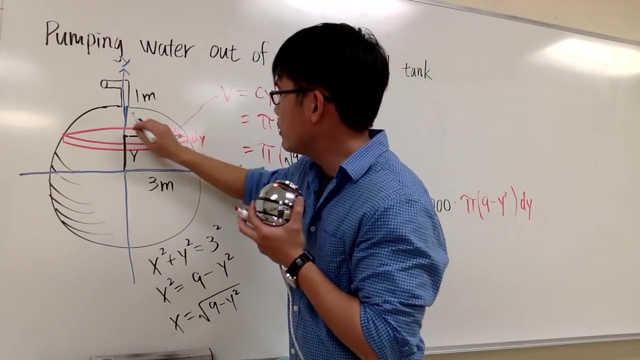 but then i need to figure out the distance travel from this disk, from here all the way out. this right here is three, so this right here will also be three, because that's also radius. this right here is already y, so this part right here in blue, and just emphasize this part. 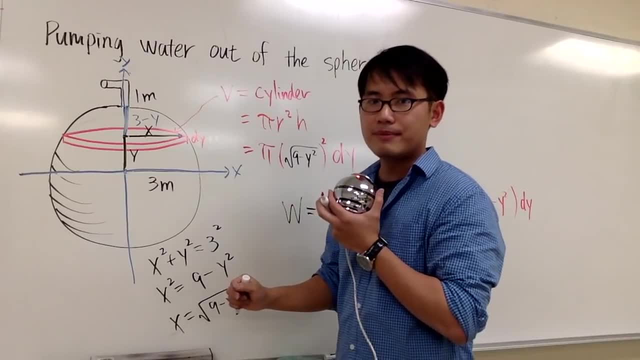 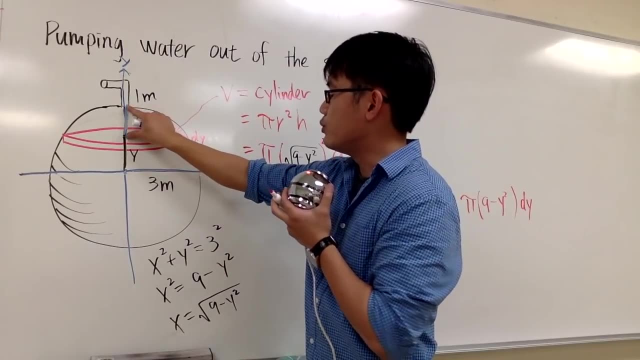 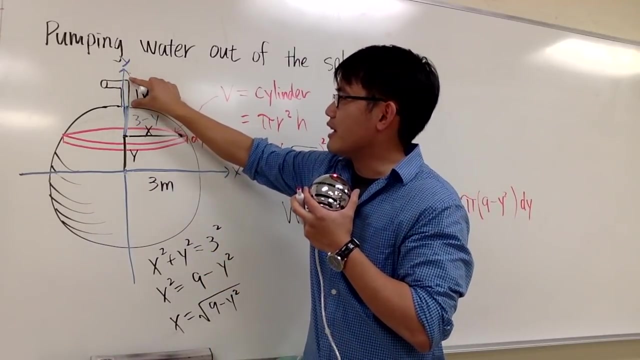 it has to be three minus y, isn't it? because once again this whole thing is equal to three, and then this much already is y already. so the remaining part is three minus y, but then you have to travel one meter extra because you have this extra thing on the top, so the 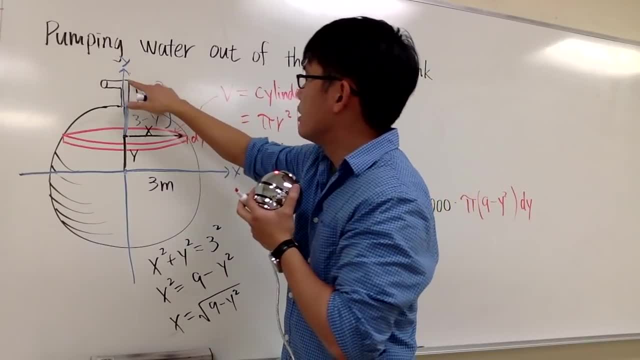 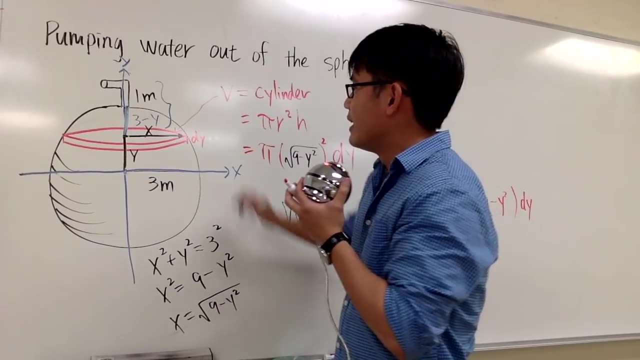 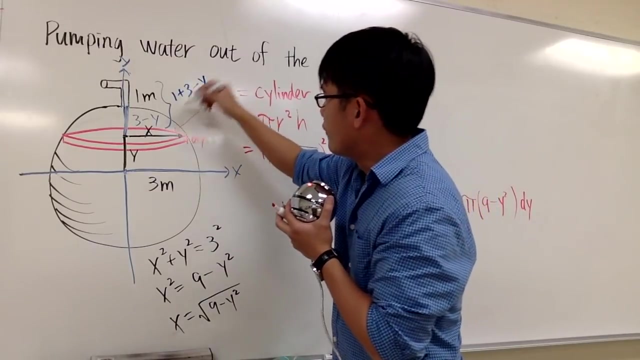 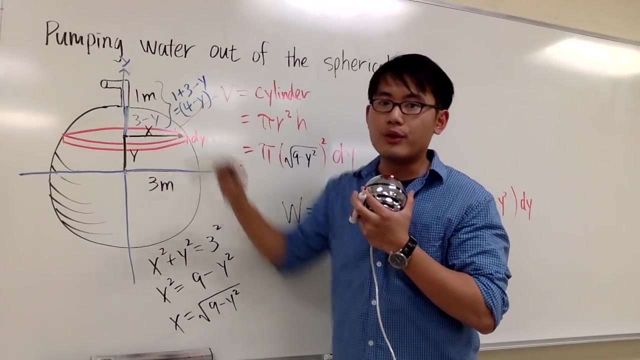 whole distance. let me just do it right here, from here, from from here all the way to the top, is what it will be: one plus three minus y, okay, and of course you can write this as four minus y, and that's the distance that this slice has to travel in order to be out. 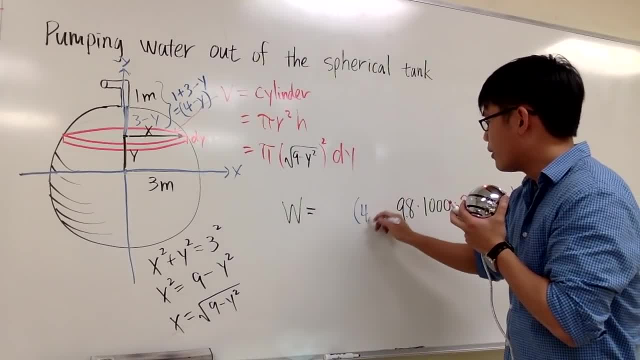 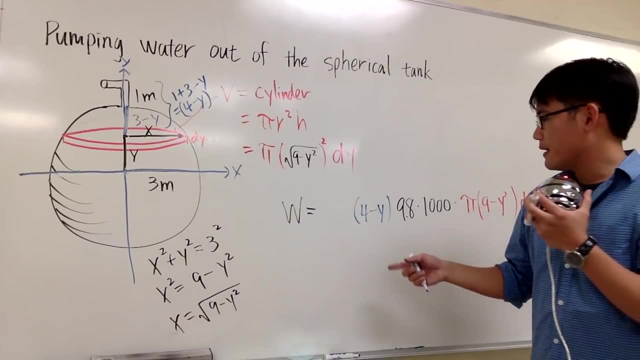 all right. so i'm going to just put this down right here: four minus y, that's a distance that it has to travel. if you look at the answer, uh solutions they have like y minus four. well, i mean like i think, y plus four, but then they just have a different coordinate system. 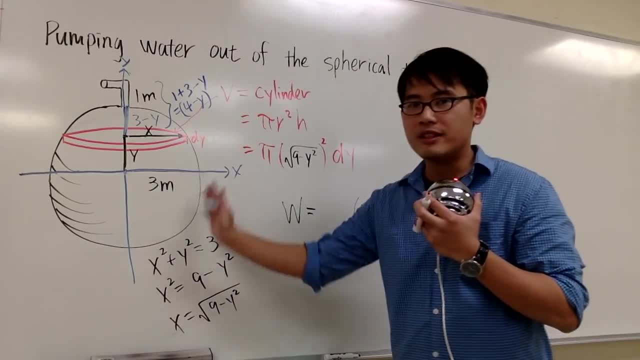 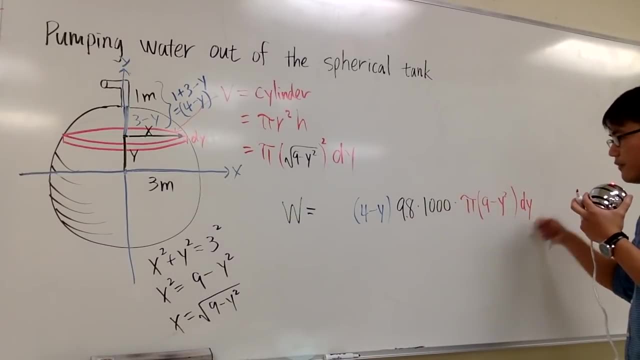 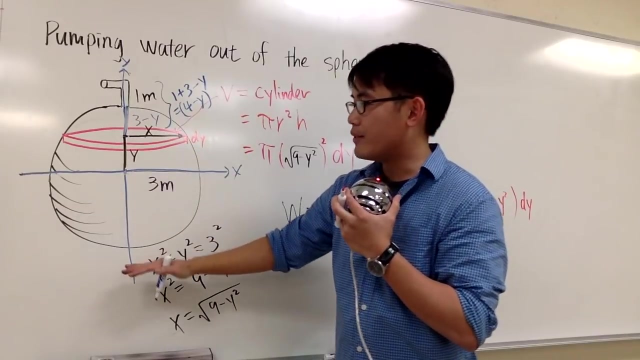 this is, uh, just as fine, because the way we set it up is just depending on, um, the different labeling. anyways, this right here is once again the force, this right here is the distance, but that was only for this slice of the, uh, the water i have to integrate now so i can find out the total work. 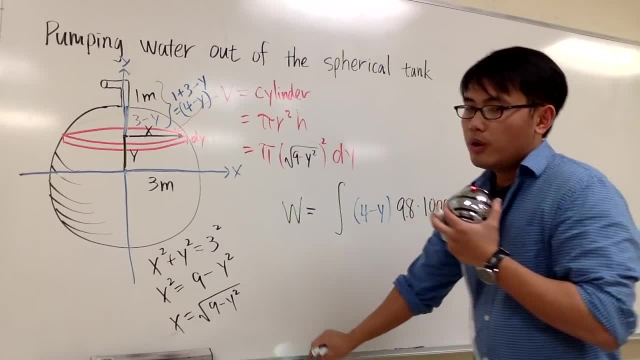 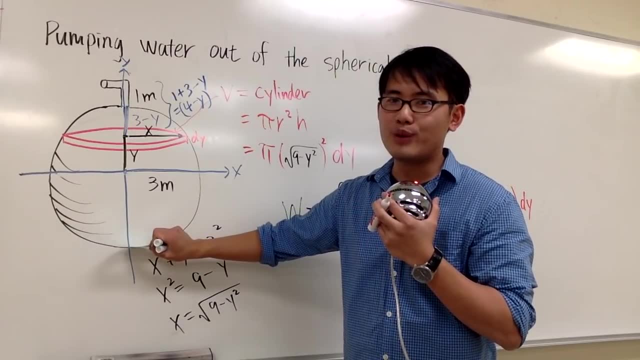 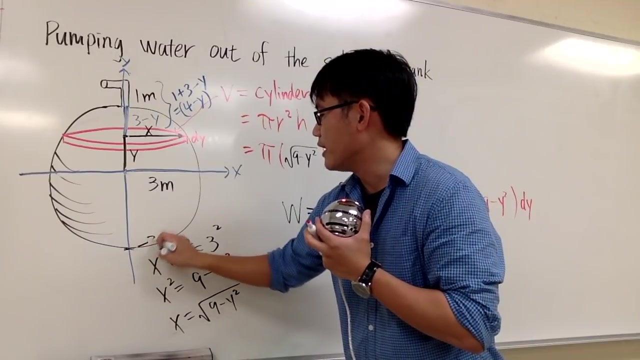 that we need. so integration will. what's the first ever cd that we have in this picture? it should be all the way down here, isn't it? and what's the beginning? y value that the radius was three down here. this power here. of course, that will be negative three, so we'll start. 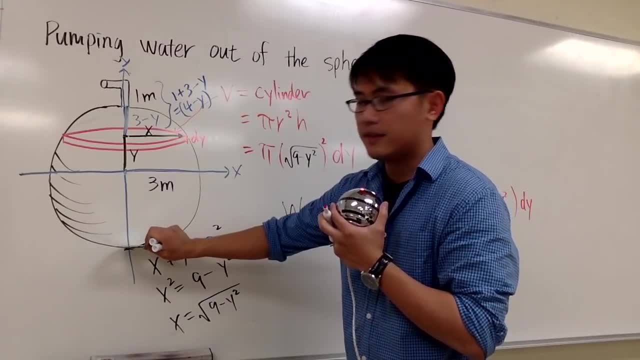 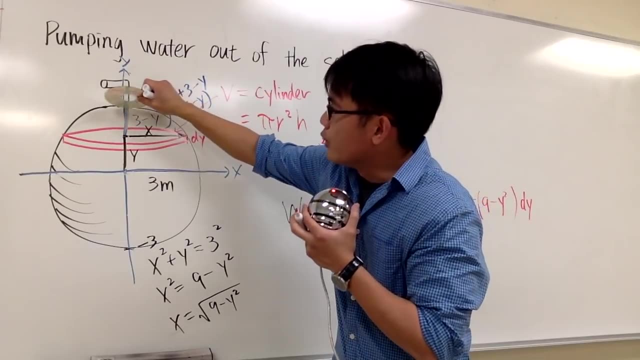